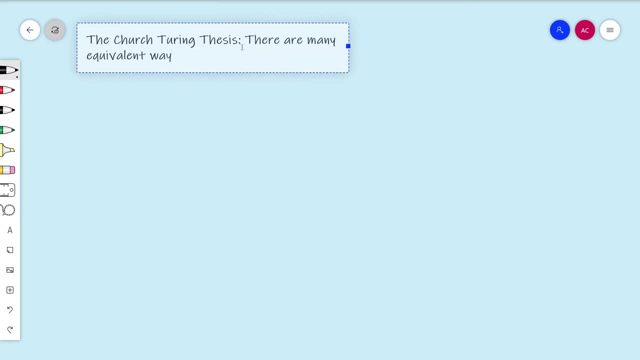 There are many equivalent ways to word this And I'm not sure really what the best one is. I think the best way to word this is all of these ways. So by model of computation, Uh, we mean, you know, a well understood apparatus for describing a deterministic machine which computes something. 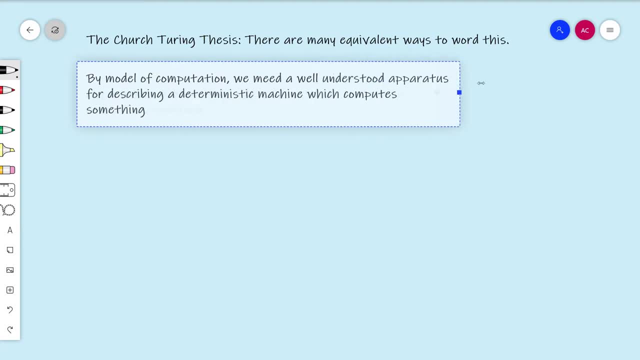 Right. I mean it's hard to define a model of computation. There is no fixed definition of what a model of computation is. We define computable. You know what we want to do is define computable. We define computable by setting some rules. you know which kind of constitute the model. 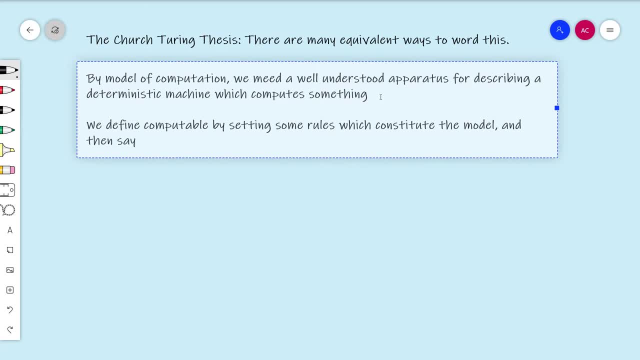 And then saying that a function or problem is computable. So if the uh, If the if, if it's computable within the model, If it can be implemented- uh, within the model. So I mean a theoretical model of computation. there's more, there's tons of options. 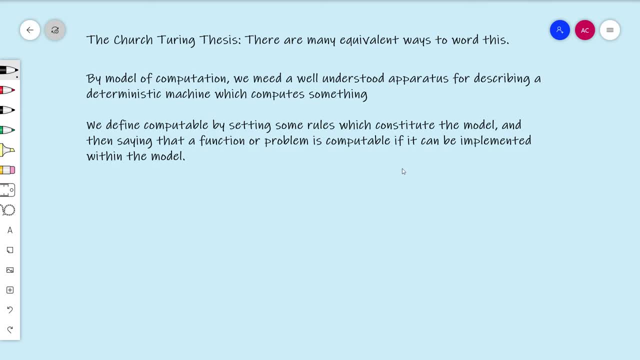 For example, you know, take your favorite programming language, That is technically a theoretical model of computation. You know if, if you know C, C, you know C programming. You've got a, you've got a language. 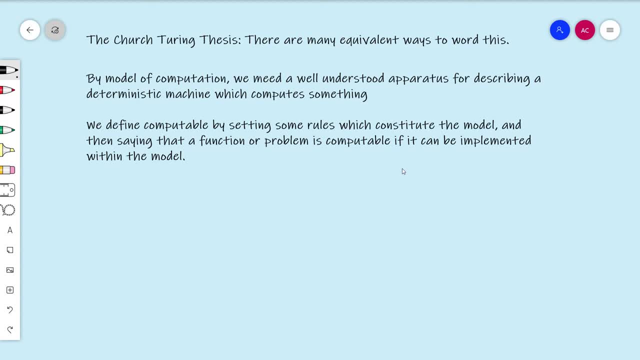 You're allowed to write. you know finite programs. You write a program in And, and basically you can say: you know a function is computable if I can write a, a program in C that does it for me, And and that's just. that's just as much of a definition of computable as our Turing machine definition. 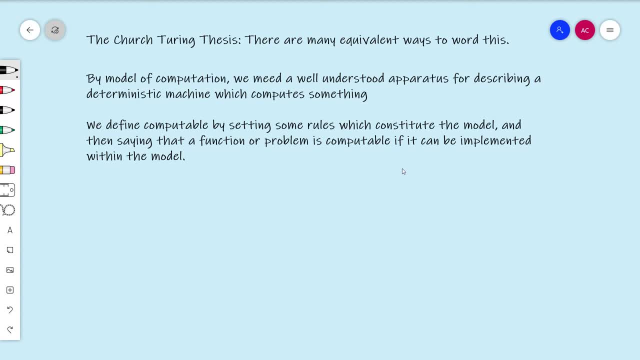 And that's the same for any any programming language. Um, so there's tons and tons and tons of models of computation And it's not really like a, a, a fixed definition, It's not really like. there's not like one kind of object that gives you a model of computation, even. 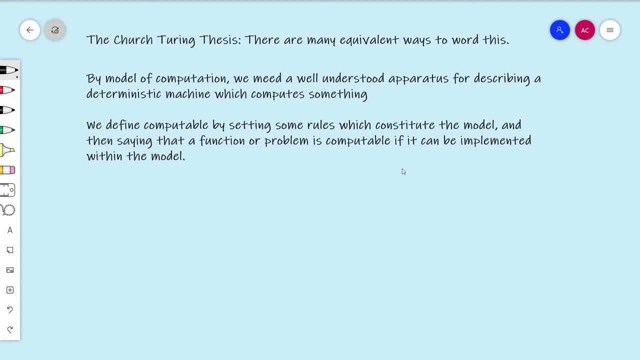 Um, so this is not a theorem: It it's, it's a, it's a statement of kind of, It's an assertion, It's a philosophical assertion, Um, and and basically it's. there's a lot of ways to state it. 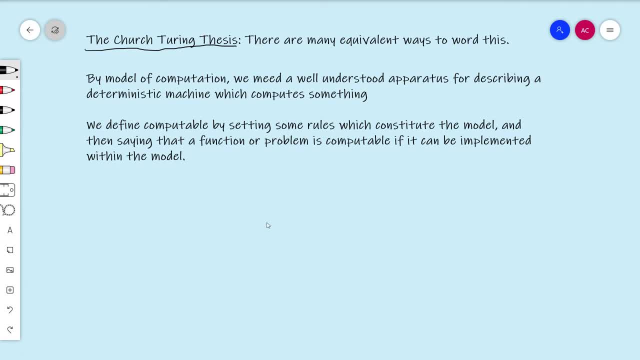 But maybe one way to state it, state it is this right, If I define computable by, it can be implemented within the model. So I can say: you know, call a function computable if it can be implemented in Java, Call a function computable if there's a Turing machine that decides it. 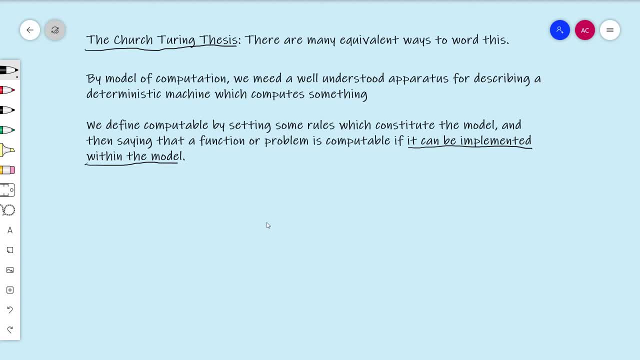 Call a function computable if there's a formula you can write out in, like the lambda calculus for it. There's a lot of ways. There's a lot of ways to say this, But you know um, But we can always define the class R. 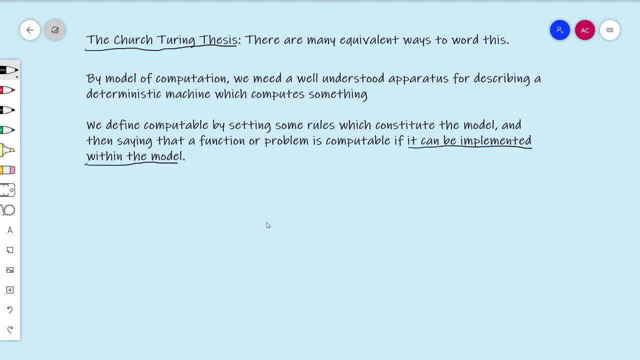 We can always define Right. the bottom line is that we spell out a model of computation and then we say it's computable if it can be implemented within the model. That's what we say. So I can always define computable, kind of in this way. 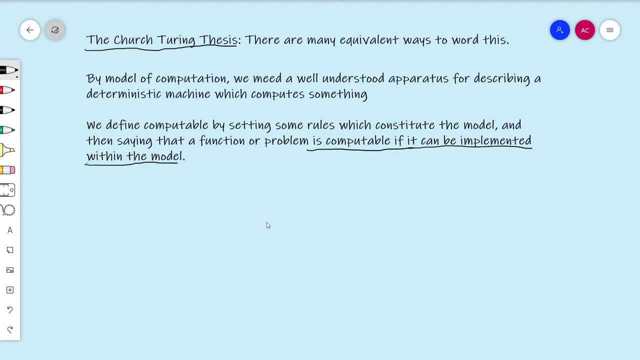 No matter what I'm talking about, No matter what my model is, I can say it's computable if it can be implemented within the model, And so I can always define The set of all computable functions, Of all computable problems. 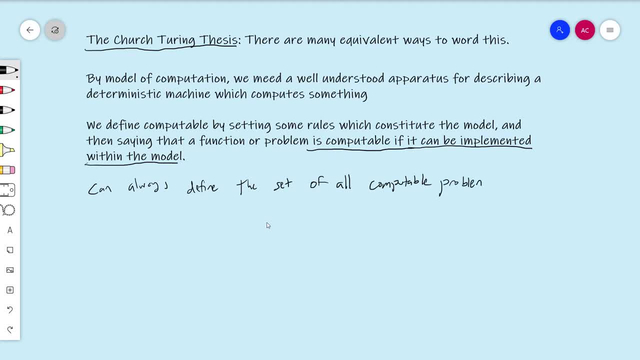 We'll show later. you know we'll justify later why the set of all computable functions is more or less the same as the set of all computable problems. Call it R. So one way to state the Church-Turing thesis Is to basically say R is the same set. 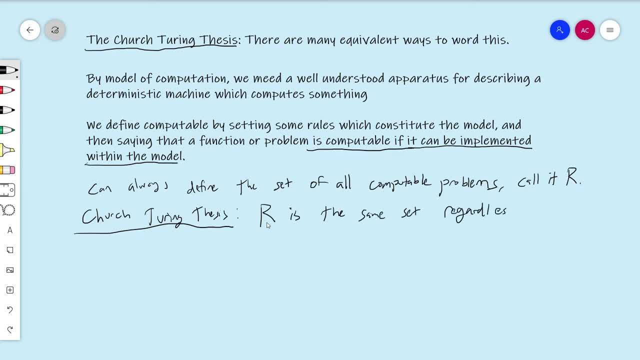 Regardless of the model. That's one way to say it. In other words, the set of all computable problems is the same set, Regardless of what's going on. Another way is to kind of take a fixed point, Like a fixed model of computation. 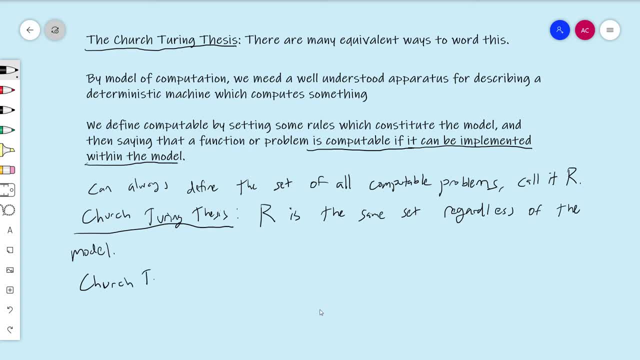 And say it's the best. Another. You know, I'll call this, I'll label this the first one. This is one way to say the Church-Turing thesis. Another way to say the Church-Turing thesis Is to say: 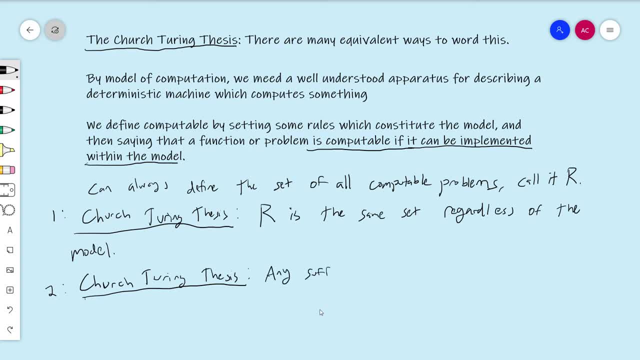 Any sufficiently A sufficiently sophisticated Model of computation Is exactly as powerful as a Turing machine. That's maybe the way to say it for us, right, Because we've been developing the Turing machine model. So any sufficiently sophisticated- There's weaker models of computation. 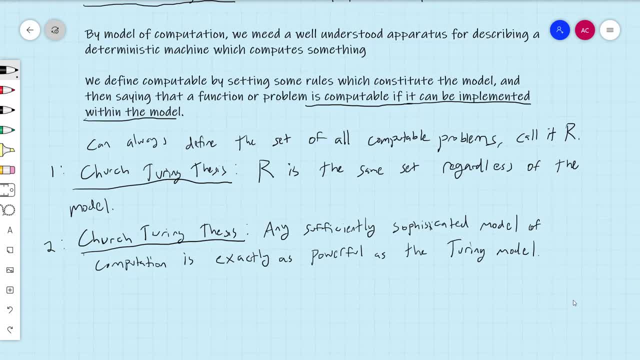 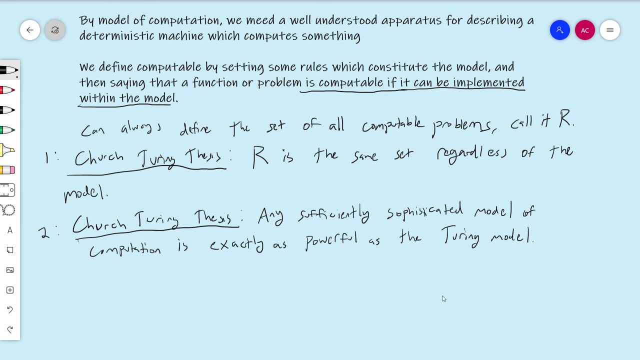 We can talk about. You know, there's push-down automata, There's finite state machines, There's models of computation that are weaker than the Turing machine model. But if you have a sufficient, If you have a good enough model, If you have a sufficiently sophisticated model, 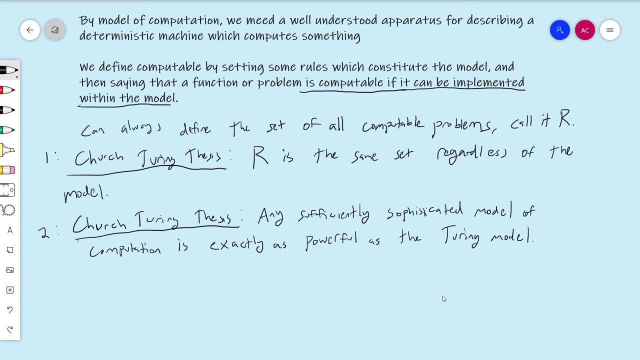 Then you know, the Church-Turing thesis can be defined as the assertion That it's no more powerful than the Turing machine model. It's exactly the same. That's one way. That's a second way to say it, A third way to say it. 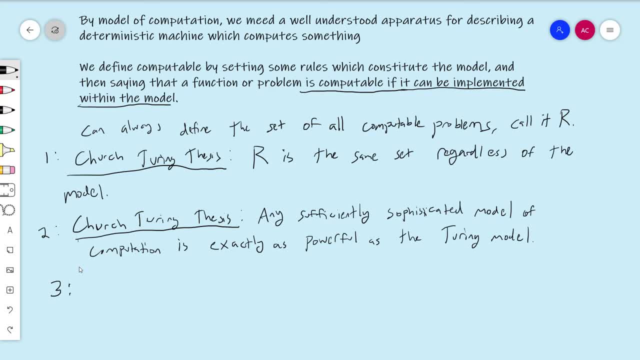 A third way to say it Is to kind of take the opposite approach. You know, over here With the second statement We sort of define the Turing model as kind of the central model. We can have kind of a completely decentralized statement of the Church-Turing thesis. 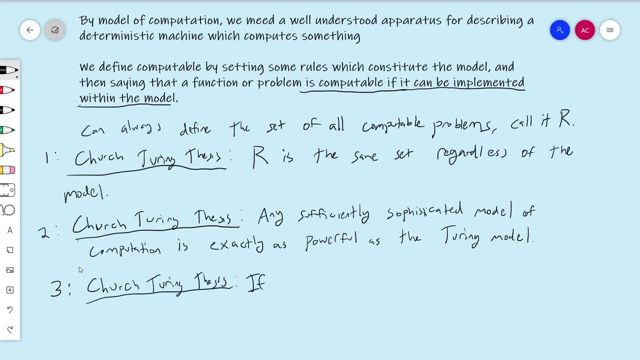 By kind of saying, If I can describe An algorithm For solving the problem, Then there's implicitly a model there, You know, Within some implicit model. It doesn't even matter. I mean, you don't even really need to make it that formal. 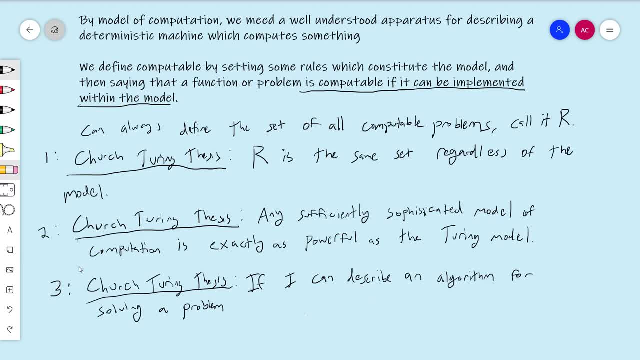 It's sort of: you know, If I can describe an algorithm for solving a problem, Then it's computable. You can take this kind of decentralized kind of setup and basically say: You know If I can do it, If I can kind of come up with a mechanical process that solves the problem. 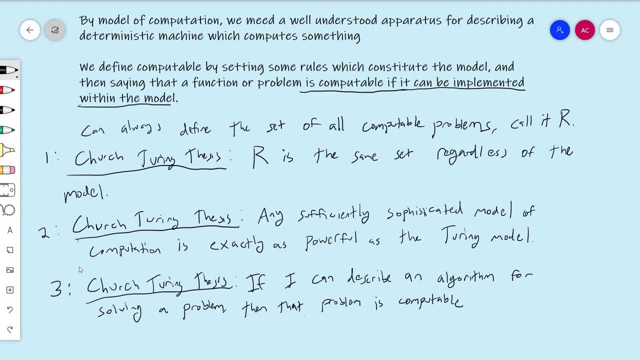 Then the problem is computable Because there's some natural model for that process that I described When I, If I describe an algorithm for something, there's implicitly a model there, And so that model is as powerful as a Turing machine, And so that problem is computable. 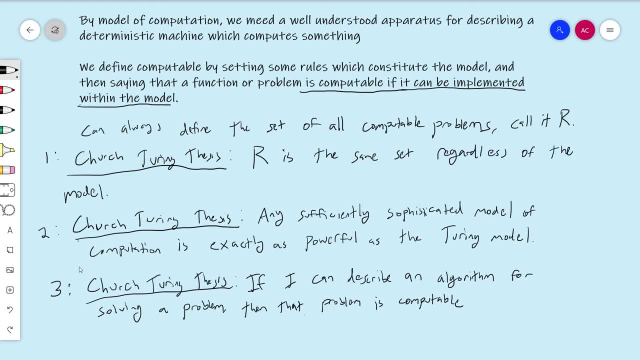 So I can kind of, You know, I can take the Church-Turing thesis and basically use it to centralize my theory. I can use it to centralize my theory. I can use it to centralize my theory around the Turing machine model. 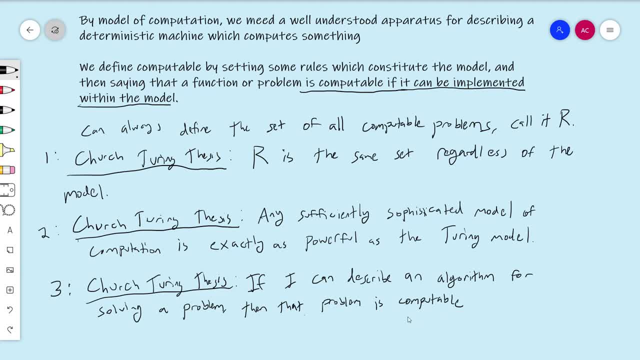 Or I can use it to completely decentralize the theory from any model And I can say: Okay, the model doesn't matter, And if I can describe an algorithm for it, then it's computable. And this is kind of a crazy statement. 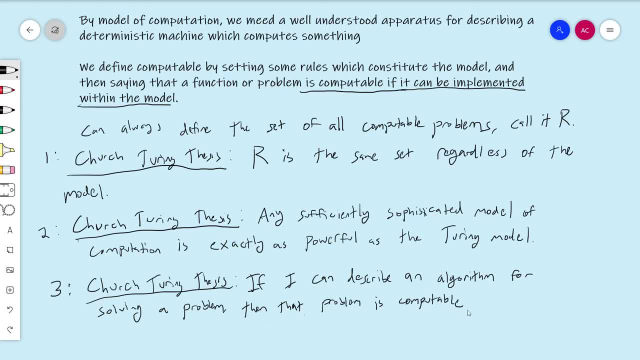 Because it essentially says that nothing we've done so far matters. Now that's not true. You know We need some fixed model to talk rigorously about stuff. But you know You can kind of get the sense from this that the model does not matter. 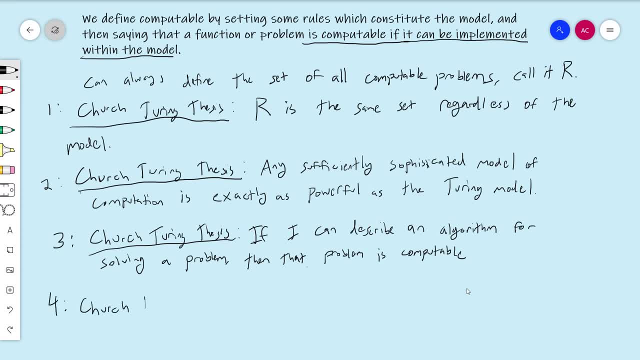 Maybe the fourth way to say it Is that the model does not matter. And so you know, There's more than even this, There's a lot of, There's still more ways to say, To talk about the Church-Turing thesis. 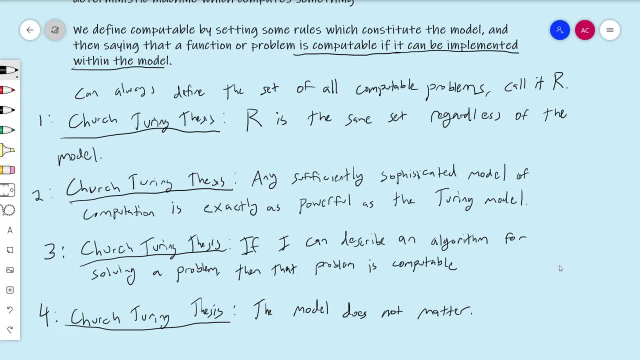 But you get the idea. The Church-Turing thesis is a statement. It's an assertion about the equivalence between all of these different parts of the model And it's a statement Between all of these different possible models of computation that anyone could ever come up with. 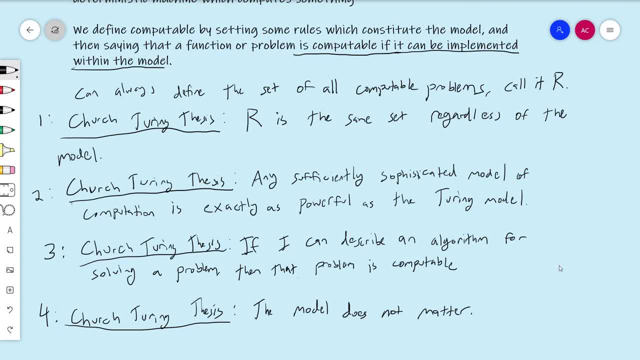 And You know there's no. There's no proof of the Church-Turing thesis. There's no fixed way to justify it completely, But the more you do stuff, the more you see it, And so that's one of the reasons why we went through all those robustness facts. 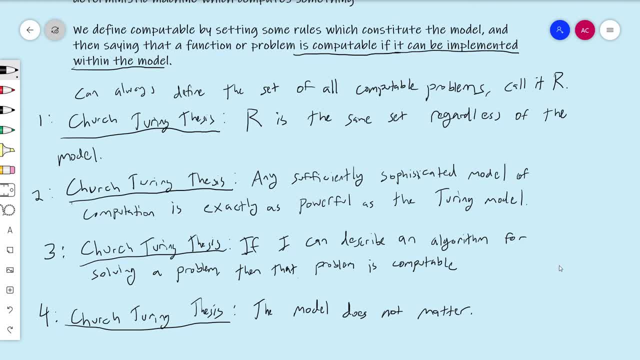 We kept doing, We kept making edits to our Turing machine model And no matter what we did, it never got any more powerful. And I even started kind of- And since it's based off that natural graph paper thing, You know the Church-Turing thesis- 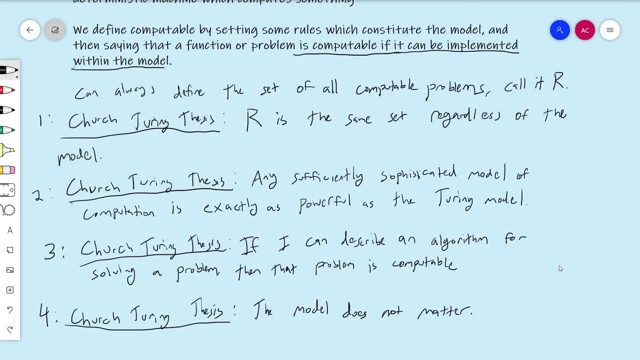 You know, the Turing model is the natural one, in the sense that It kind of naturally relates to a person doing something on paper And that's kind of what. So that maybe connects to this third one here, And I even invoked that a few times when I was building my 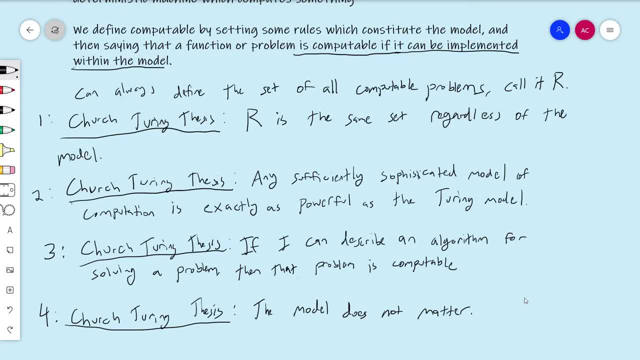 My universal Turing machine. I said, alright, logarithms, I don't care about logarithms right now, I can do those on paper. Since I can do a logarithm on paper, I can do it. I can do it on. 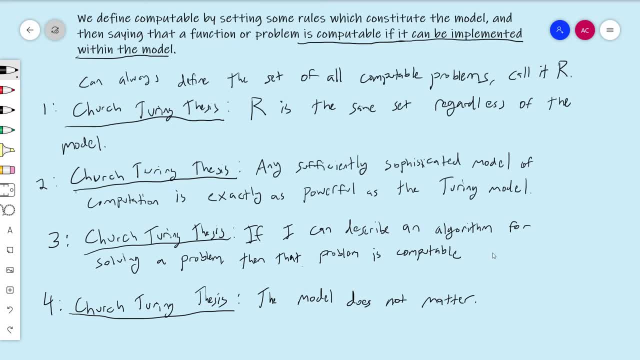 I can do it via the Church-Turing thesis, The Church-Turing thesis on a Turing machine. That's sort of an invo. That's sort of like a lesser invocation of the Church-Turing thesis. So The Church-Turing thesis is sort of a centraling. 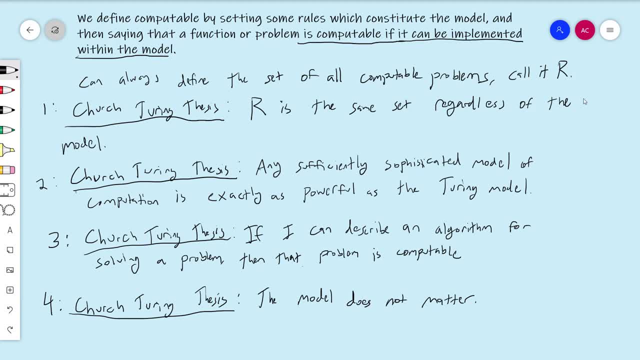 A central, like philosophical thing that we need to make sure that we are aware of before proceeding forward. It basically says that the model that we've developed, While it is valuable in terms of having a rigorous idea of what we're going to be talking about from here on, 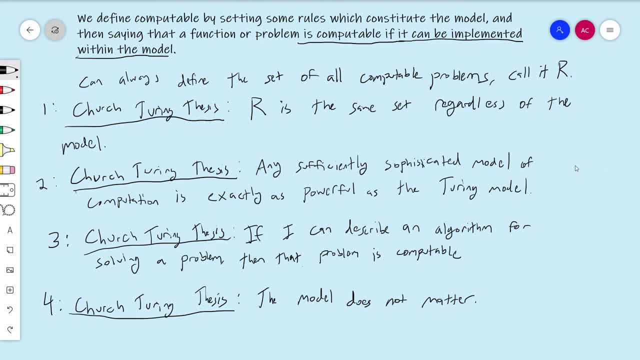 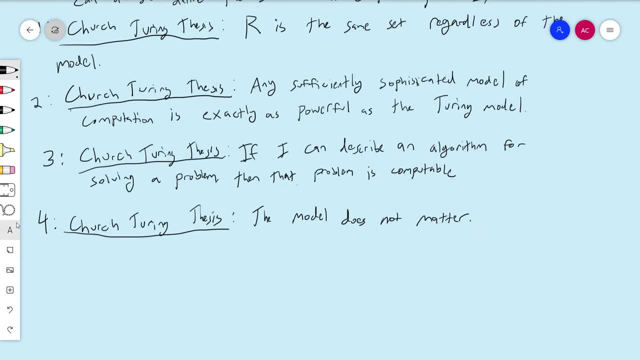 We're talking more or less about. When we talk about computability, We're talking about far more than just Turing machines. Maybe I'll write that down: Um, The Church-Turing thesis Confirms That when we are proving facts about Turing machines, 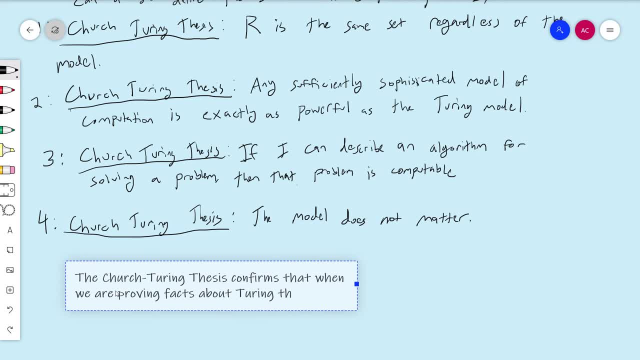 Uh, We are proving facts about computability in general, So all of these are going to be important to note. You know, I can invoke the Church-Turing thesis by describing a mechanical algorithm for solving a problem without actually giving you a Turing machine for it. 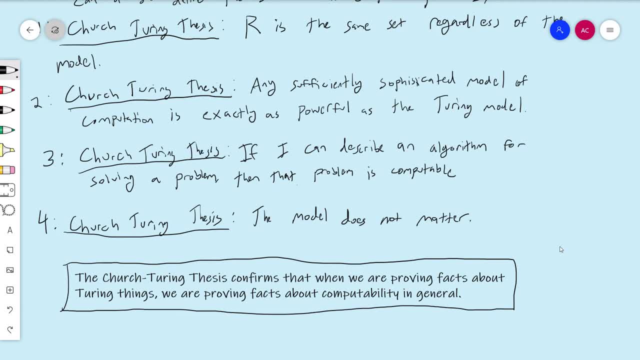 We'll do. You know, that's the thing that people really hate about computability theory, Like the people that are real sticklers for mathematical rigor and like justification, And so we'll use that as little as possible. But it's almost impossible to completely avoid using the Church-Turing thesis sometimes in that regard. 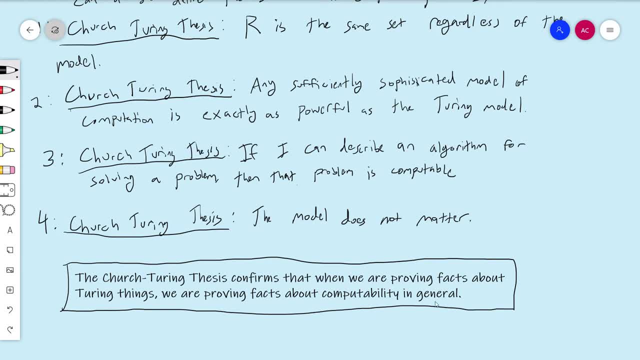 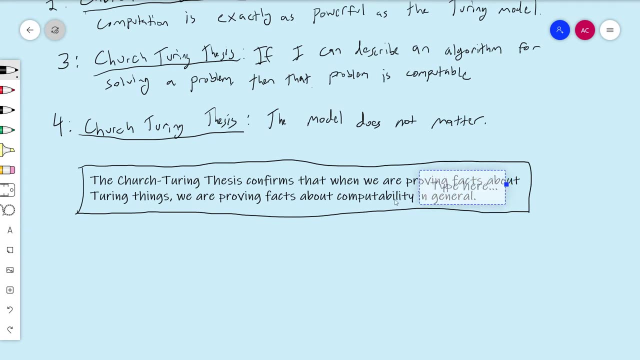 But even beyond that, It sort of also matters in the sense that, You know, it confirms that what we're going to be doing in the future Is Relates to far more than just Turing machines. Um, One last thing: The strong Church-Turing thesis. 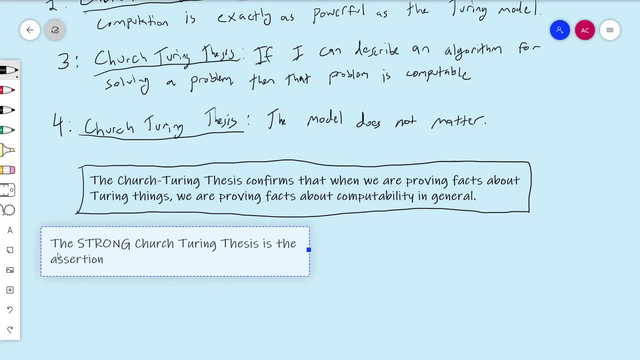 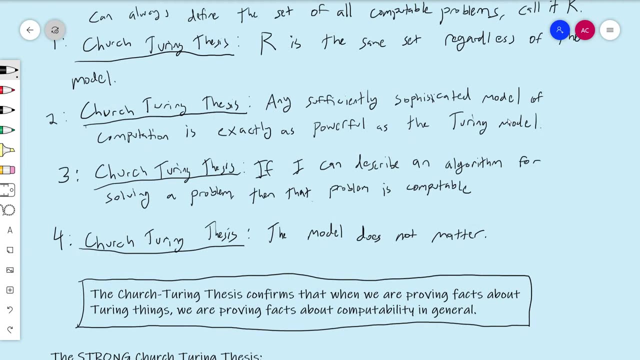 Is the assertion. Let me Is this: The easiest way to kind of think about the strong Church-Turing thesis Is to look back at the first thing I said. The Church-Turing thesis was the statement that R is the same set regardless of the model. 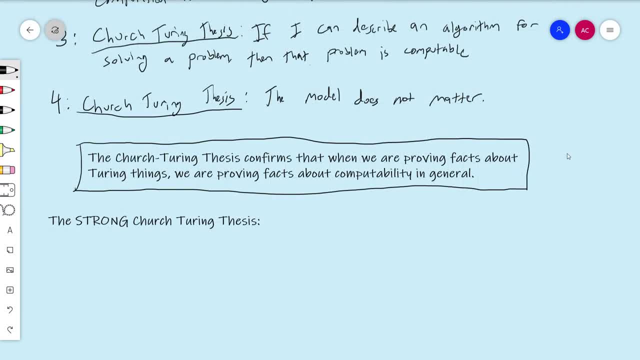 The strong Church-Turing thesis. The strong Church-Turing thesis- I'll restate this later, But the strong Church-Turing thesis- is the assertion that P is the same set, Regardless of the model. Now, what is P? P is the set of all problems that can be decided efficiently. 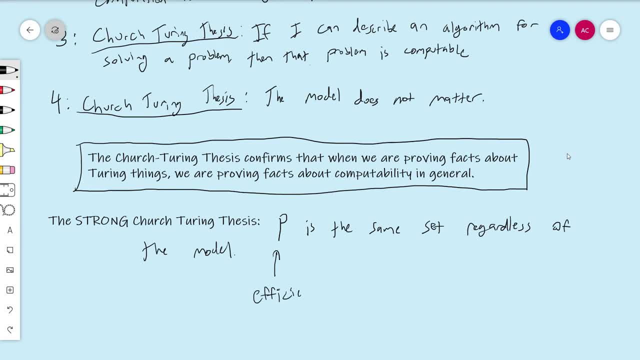 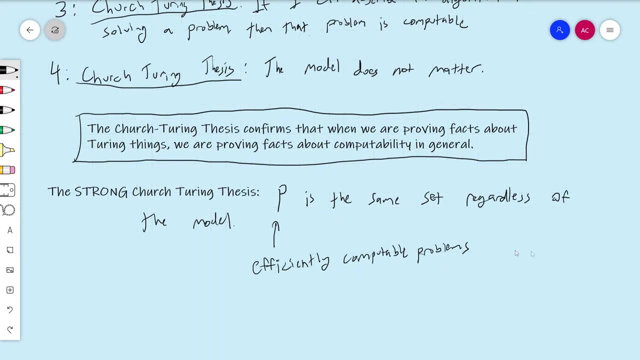 Not just computable problems, but efficiently Computable Problems. Um, Now we saw. Now we saw that two string Turing machines, Two tape Turing machines Were technically faster On some problems than one tape Turing machine, But not in a way that affects the set P. 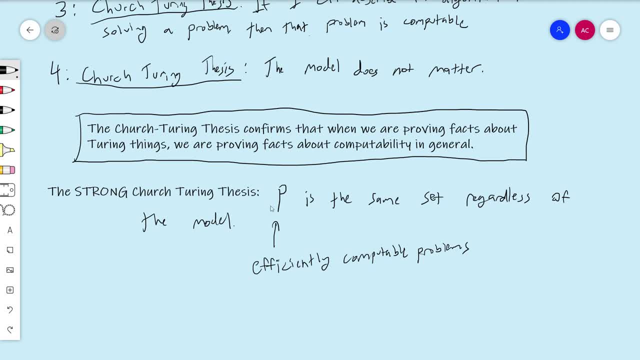 So that That doesn't challenge the strong Church-Turing thesis We're just talking about. You know, The set of decently efficient things is still decently efficient. However you define efficiency And That sort of That sort of relates to this assumption we made when we were talking about difficulty in general. 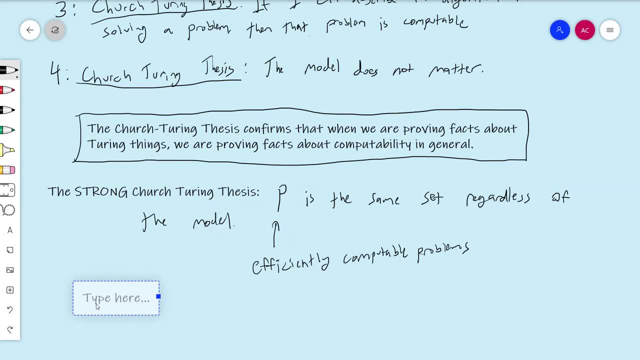 When we were talking about operationalizing our notion of difficulty by kind of defining, You know what we said before. I think was that What we said before is that if a problem is difficult, Then it will Always Consume. 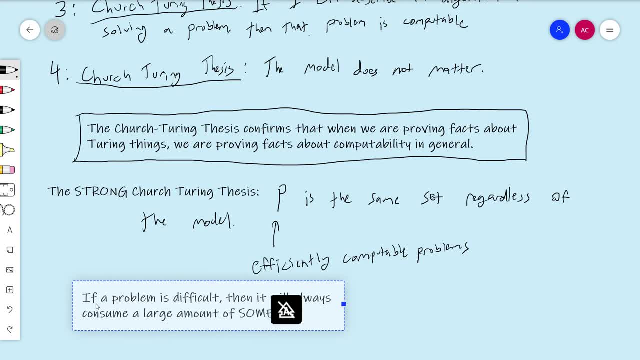 A large amount Of Some Resource, Um, In any model of computation. This was kind of the fundamental assertion that we taught, That we like started with in order to kind of justify That we can analyze the difficulty of problems via resource consumption in some model of computation. 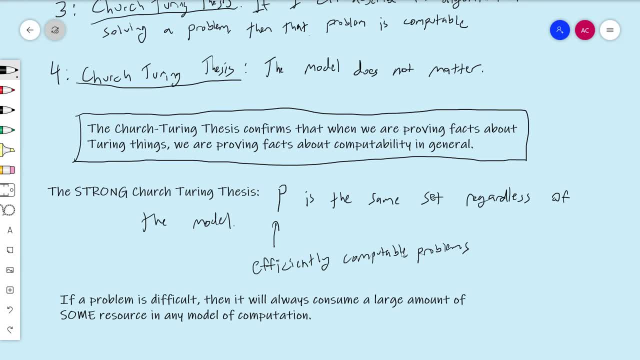 Uh, Now, You know, There's an assumption here too, that kind of Uh, That That we have some notion of time efficiency for any model. Um, And so There's, There's a lot to say here. 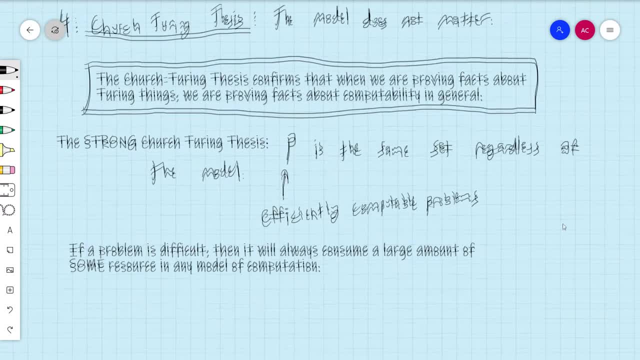 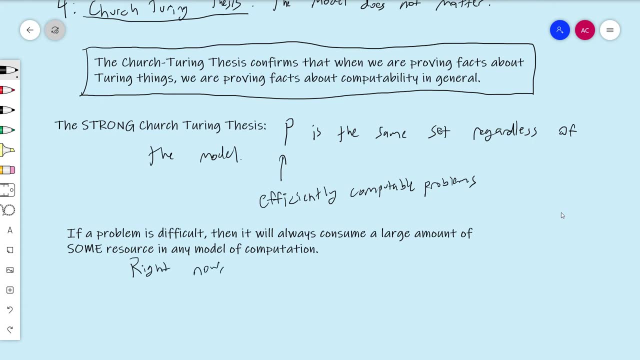 I mean, I mean this isn't going to be our full discussion of the strong tertiary thesis, But Right now, Uh, Quantum computers, Uh, Are a direct challenge To the strong tertiary thesis. That It I, I. 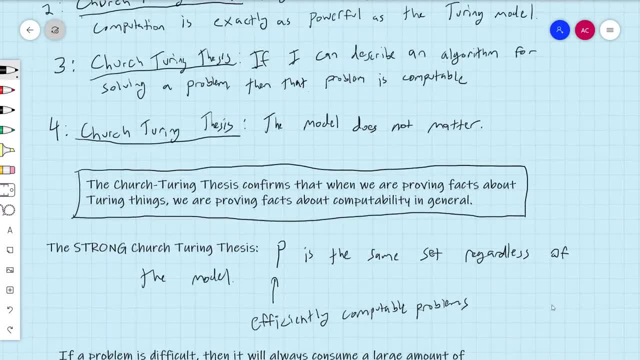 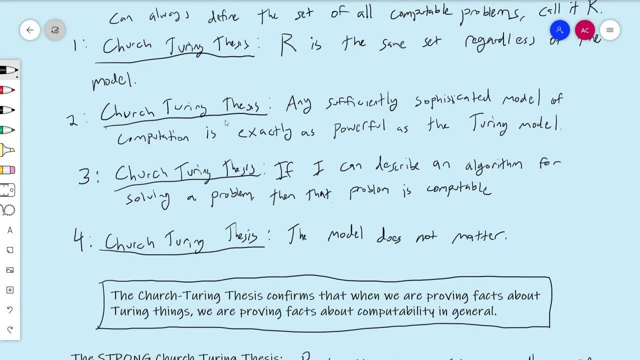 I I want people to understand this. A lot of people believe quantum computers are just magic. No, Quantum computers cannot do anything more than a Turing machine can do. We Nobody, Nobody on Earth doubts the strong. Nobody is going to denou. 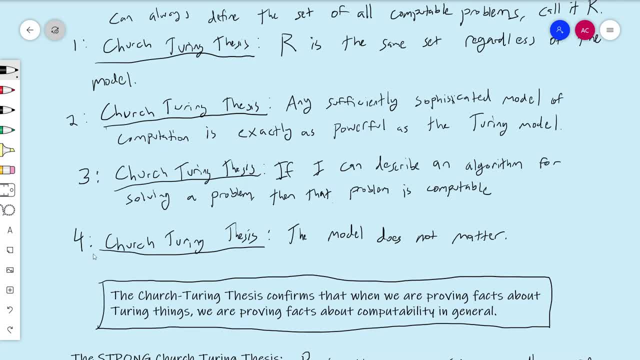 Nobody doubts the Church-Turing thesis. We still have never found a A model of computation. This, The Church-Turing thesis, deeply relates to, like what we think of as computability in general, Uh, Algorithmic processes in general, as we think of them, bound the Church-Turing thesis. 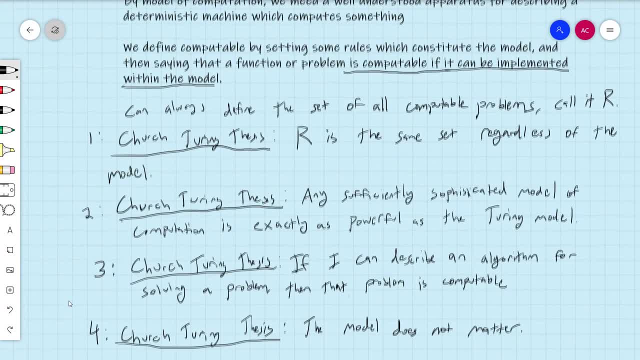 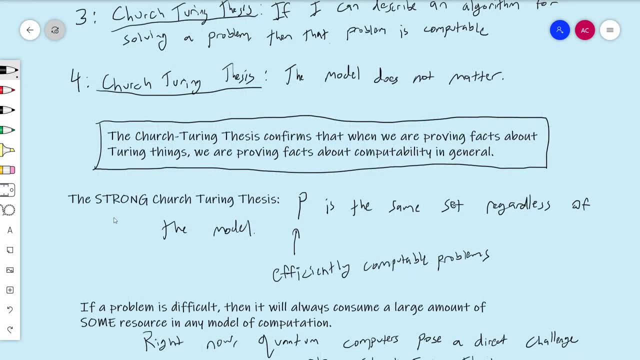 However, There's a lot of Of Uh Wiggling Kind of Going on here. This is a much less rigorous claim: Um, And And, And. so quantum computers. They pose a challenge to the strong tertiary thesis. 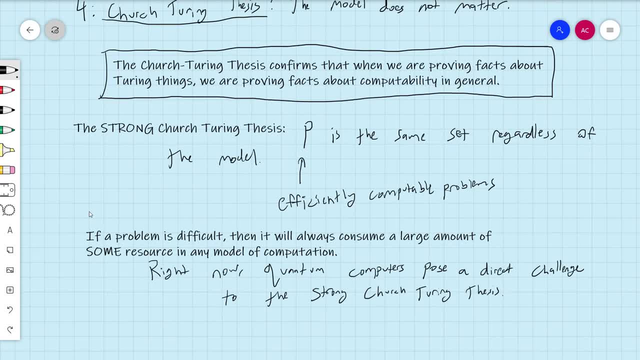 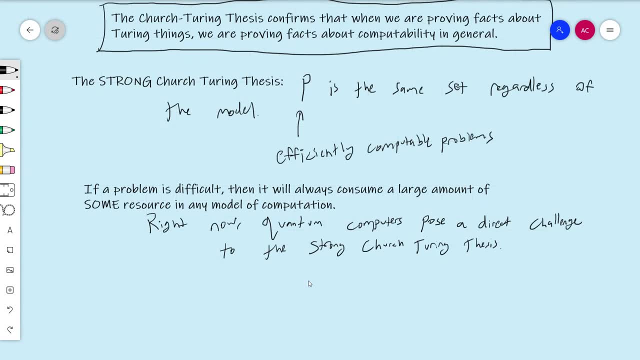 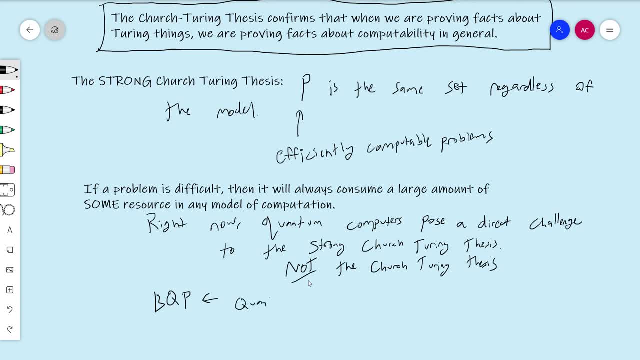 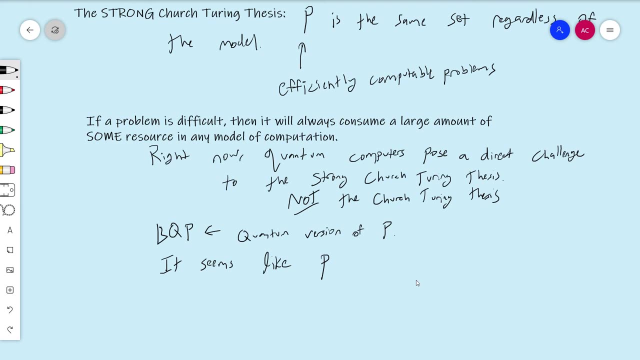 This is essentially the quantum version of P, Uh, And, And it's The case, It seems Like, Like, It's possible, Like It seems that Uh, P is strictly contained, is properly contained. It seems like P is properly contained in BQP. 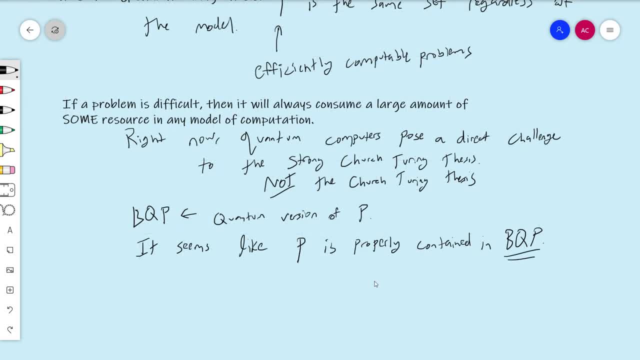 That is to say that BQP is a distinctly bigger class. Now, that's not proven, but it seems that way And in fact it is the case that if BQP is equal to P, then I believe it ends up being the case that P is equal to NP. 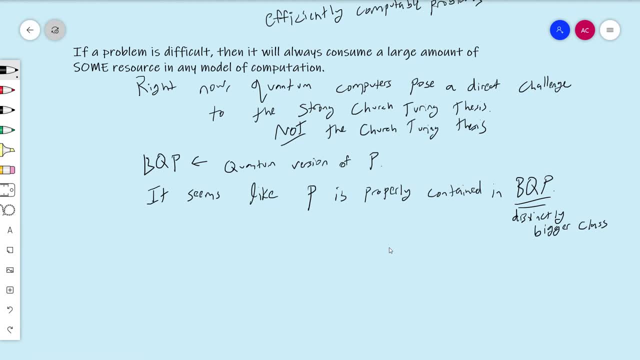 which is almost certainly not the case. So it's almost certainly the case that P is not equal to BQP. However, not only is BQP an R, BQP is actually a subset of P space, polynomial space usage. So I mean, it's really like. 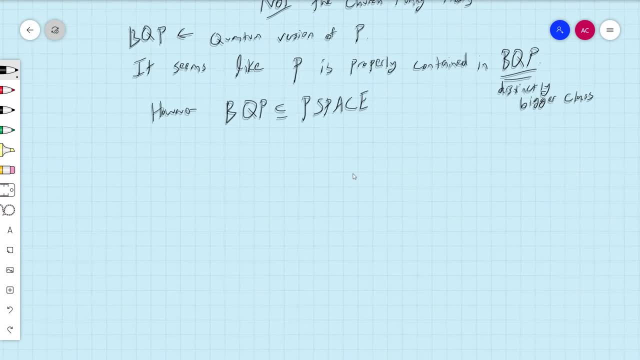 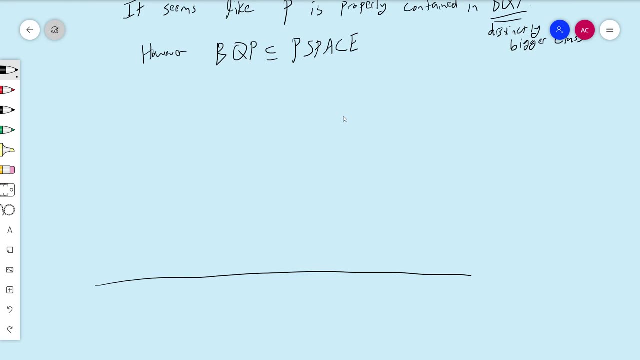 It's not a gigantic improvement. I mean it is in terms of practicality, but in terms of the big picture of what's computable, we've got P. Here's the big class of recursive function. It's gigantic. And then here's P space: baby old P space. 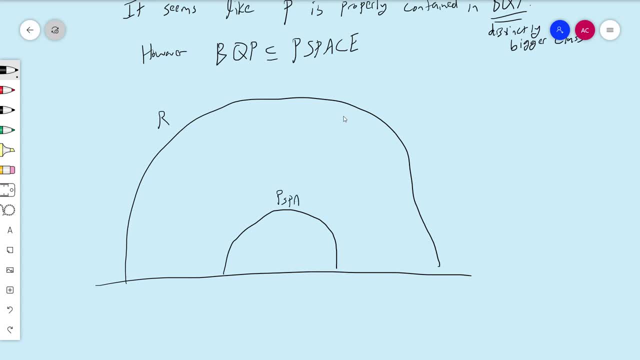 So here, this is R, This is P space, This is P. And then this is like BQP: It's not even, It's not only a subset of R, it's a subset of P space. So it's really like you know. 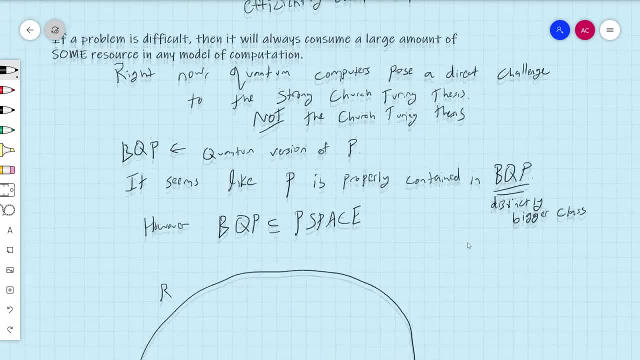 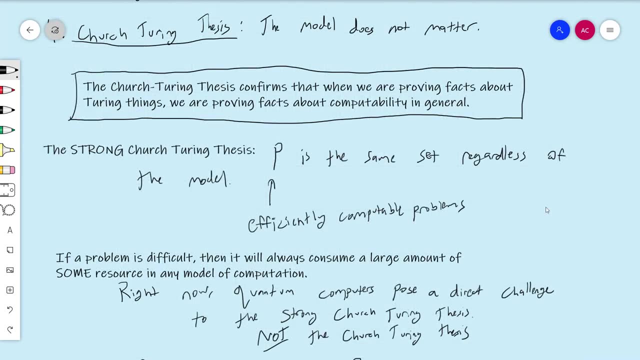 temporary expectations, I guess, is what I'm saying with regards to quantum computers. They have a lot to offer, but they're not magic, And so this is exactly where they stand right now. We'll talk more about those later, But I felt like before we move on. 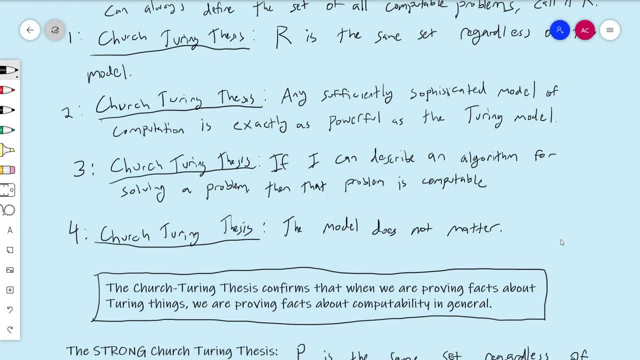 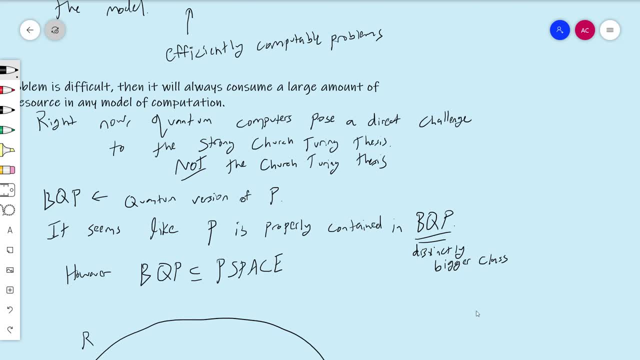 we really should kind of talk about the church-turning thesis. So that's what we did. Hi me again. I just wanted to correct myself. I said earlier in this video that If P is equal to BQP, then P also is equal to NP. 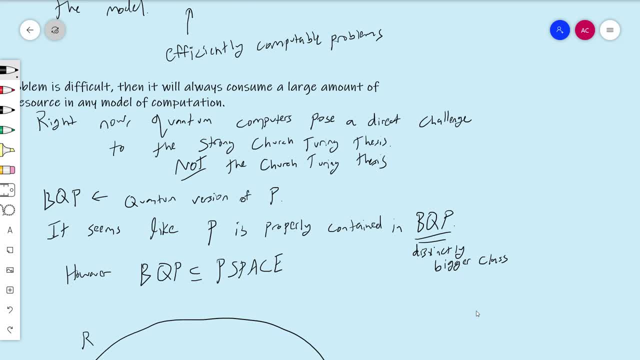 That is extremely unlikely to be the case, because it's very unlikely for various reasons, that NP is contained in BQP. But it is not necessarily- That's not a logical statement- that if P is equal to BQP, then P is also equal to NP. 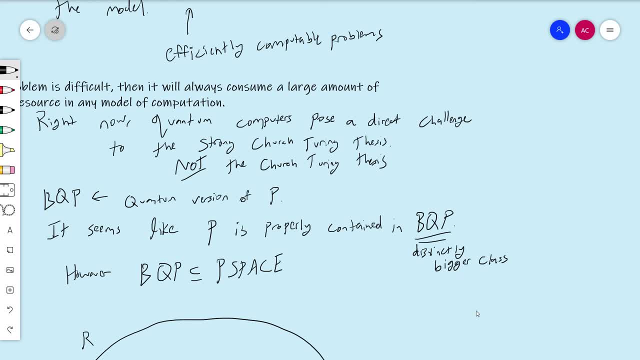 That could still be the case. It could still be the case that P is equal to BQP, but P is not equal to NP. That could still happen. Probably not, but it could, So I just wanted to correct myself.